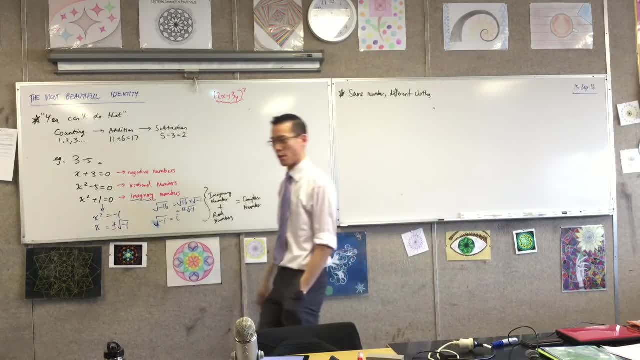 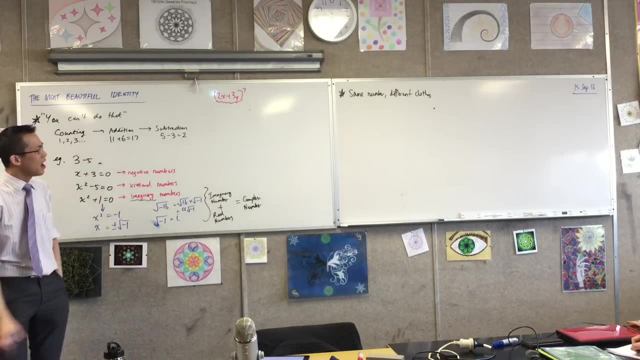 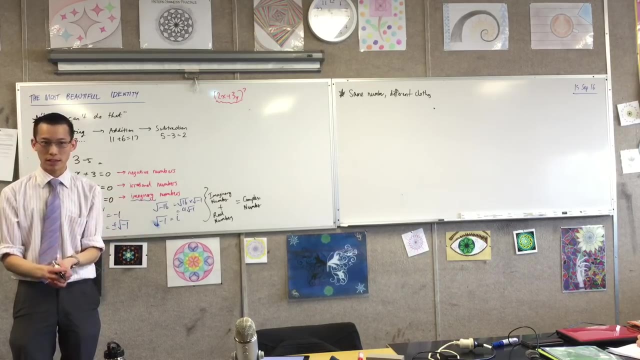 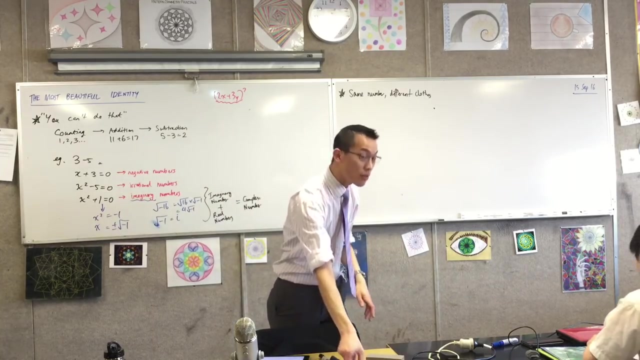 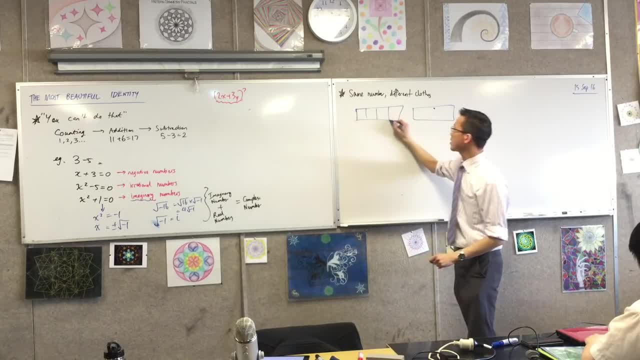 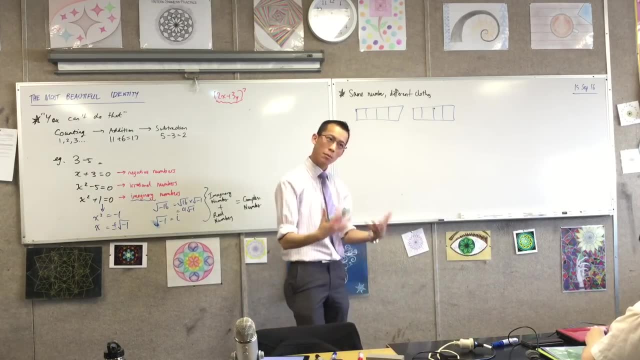 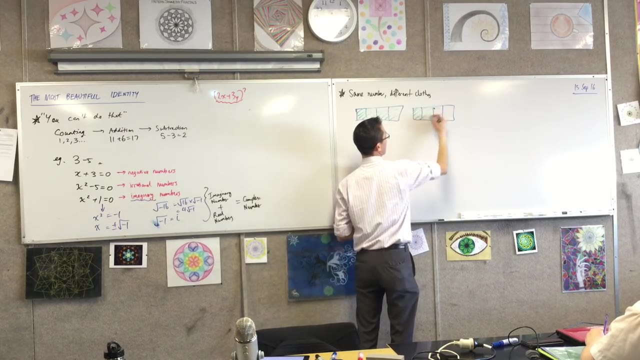 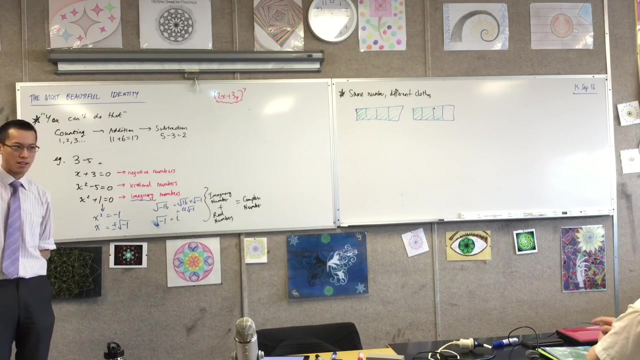 I just want you to have a look at this number and think about how you would say it. okay, I'm deliberately not using any digits, because that's kind of the point. So the number I'm going to put on there is what I'm going to shade in green. okay, So if I put this through here, Okay, now, just look at this for a moment. This is a number, okay. Now I just want you to think, think And on the count of three, I'm going to ask you all to tell me. 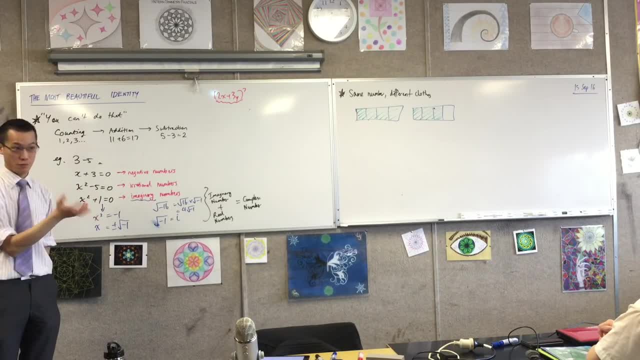 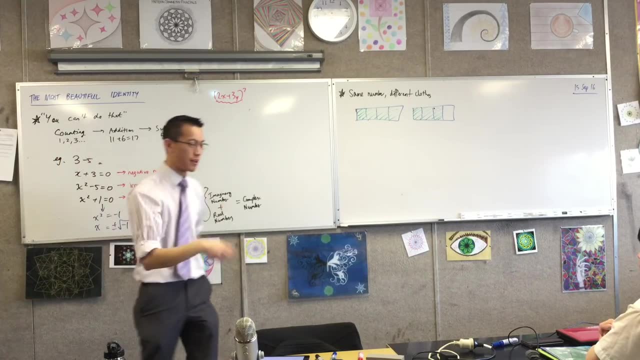 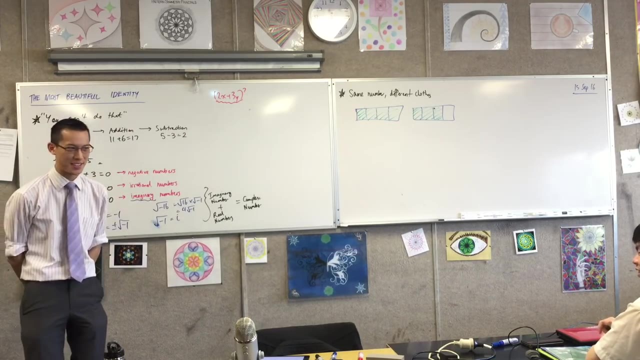 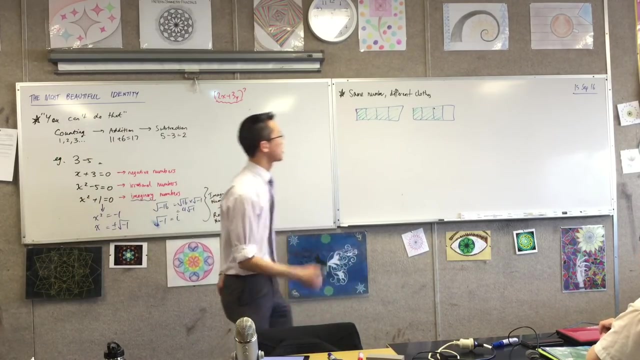 how you would say or write this number: okay, Are you ready? All at the same time. okay, That's a number. How would you say it? Ready On the count of three? One, two, three, Okay, so I heard at least three different answers. You're all at the same time so I kind of didn't quite. there were probably more. okay, I can think of at least four ways to write this number. okay, And depending on what you were thinking- because I deliberately didn't give you any sort of lead into this- depending on what you thought that represented. 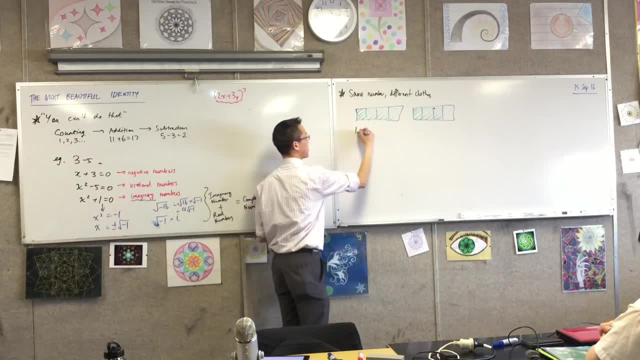 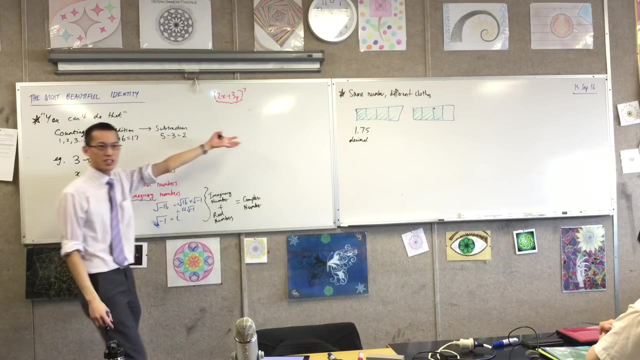 you could say that in a few different ways. Here are the ways I've got. I heard 1.75, for sure We have a name for this kind of representation. What do we call it? We call it a decimal, But you know the ancient Greeks, who dealt so much with rational numbers, they had no system for decimals, right? So I'm pretty sure I heard someone say something to do with a fraction. What did they say? 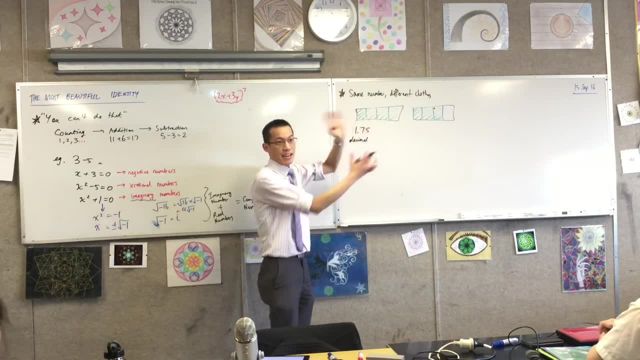 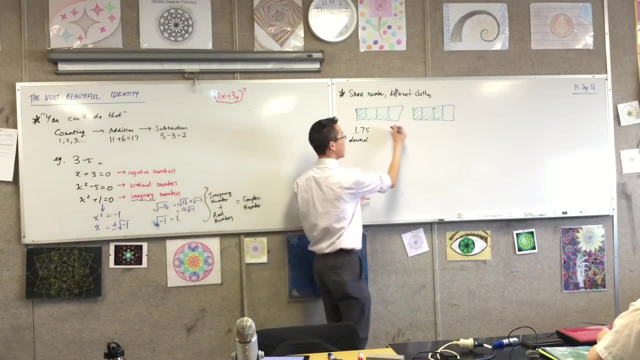 Okay, now you said seven-eighths. That's fine, because again, I didn't give you any lead in. I kind of intended these as two wholes. right, But these are a separate whole. This is really actually seven-quarters. Yes, Seven-quarters okay, Because like one, two, three, four, five, six, seven, What do we call this representation? 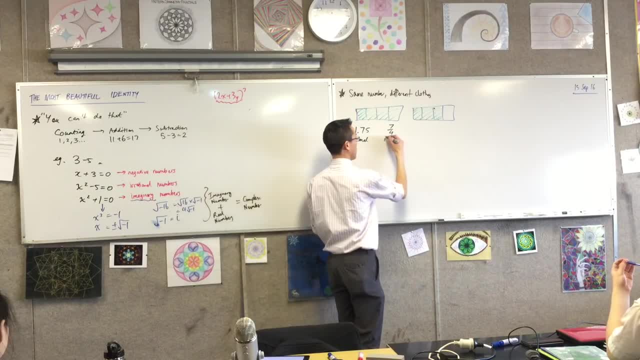 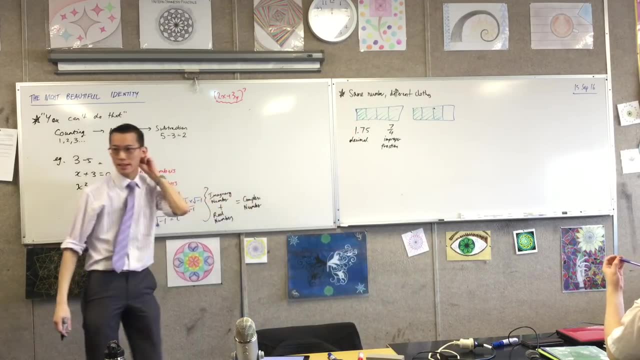 Fraction of a fraction. This is an improper fraction, right? How else? How else could I say it? I could do it as a mixed numeral, right, A mixed numeral, and I would say one and One and three-quarters, One and three-quarters right. 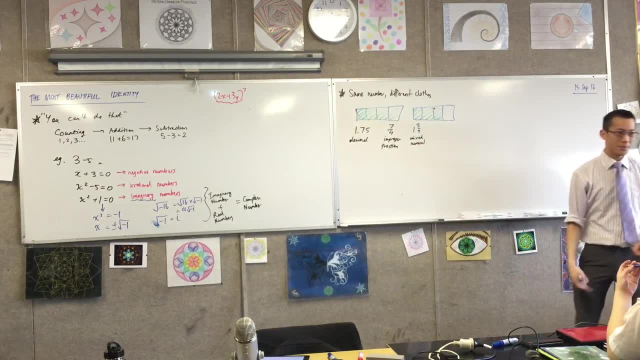 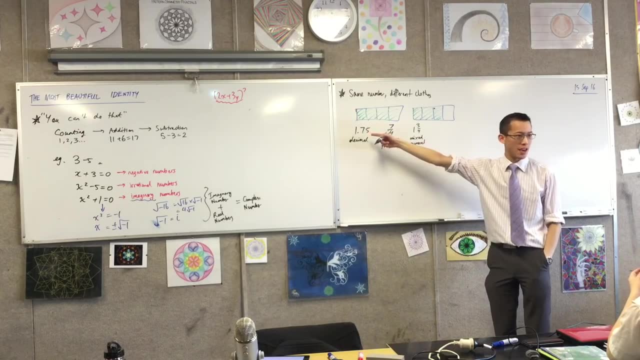 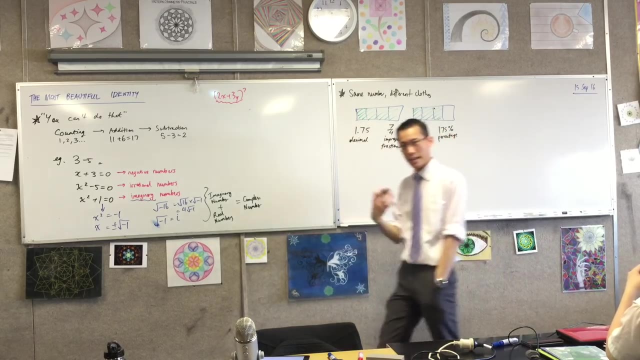 There's one more way which I can think of quickly, which is a percentage, right. So I would say this is a hundred and seventy-five percent as a percentage right Now. these are all the same number. They are just wearing different clothes and each one the reason why we've learned so many different ways of saying the same thing, like you know well. just think we have like a similar number of ways of writing this, right. 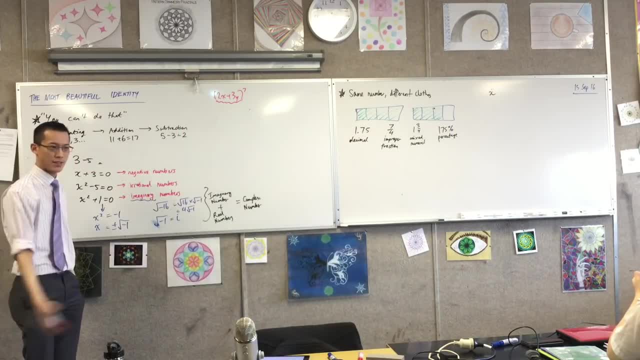 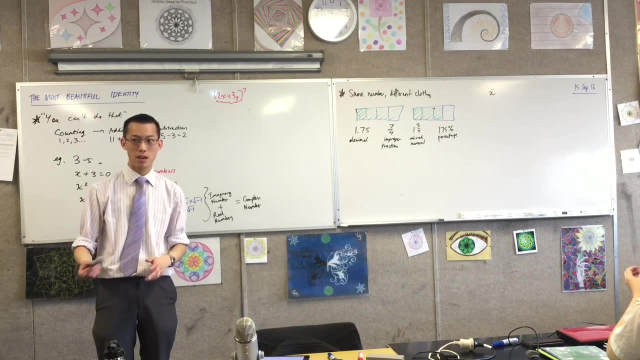 Like five right: V, T, V, D, V, L, E, X, D, R. you get the idea, okay. Why do we have so many different ways of saying the same thing? They represent different things when represented differently. 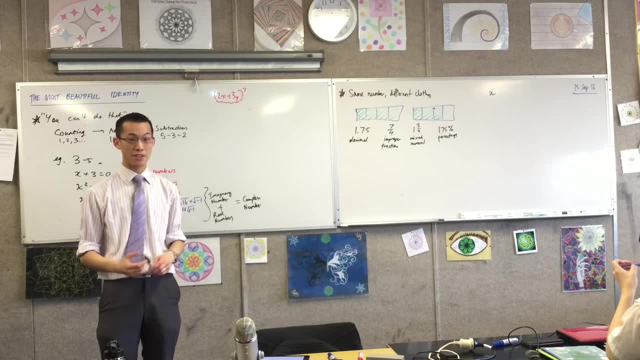 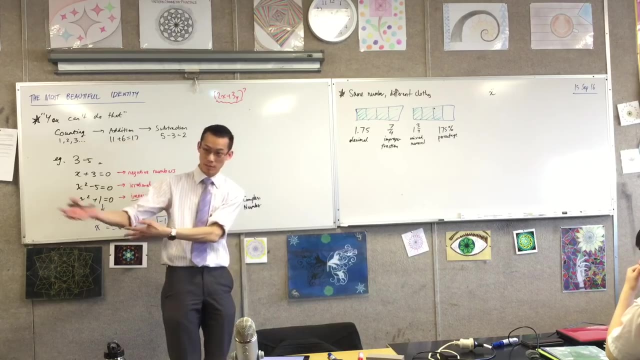 Hold on a second. Aren't they all the same thing, Aren't they all? acceleration? Well, they're all the same thing, but they've, like, worked with different numerals and different numbers to form that acceleration. Yeah, very good. So same concept, but it's like, well, tell me what you've got. Do you know stuff about velocity? Do you know stuff about displacement? Do you know stuff about time? 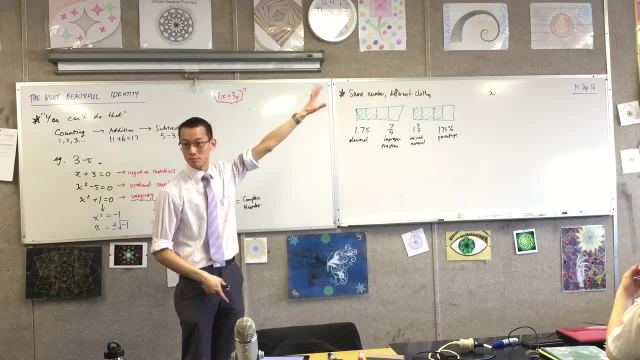 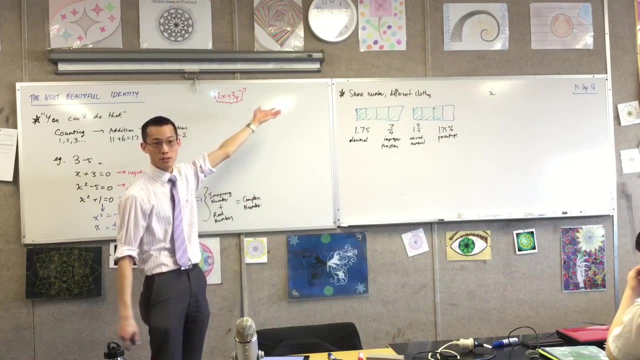 Yeah, Depending on the kind of problem you're trying to solve, you will use a different one, right. And in the same way, depending on the kind of problem you're trying to solve or the idea you're trying to express, you will use a different one of these, okay. 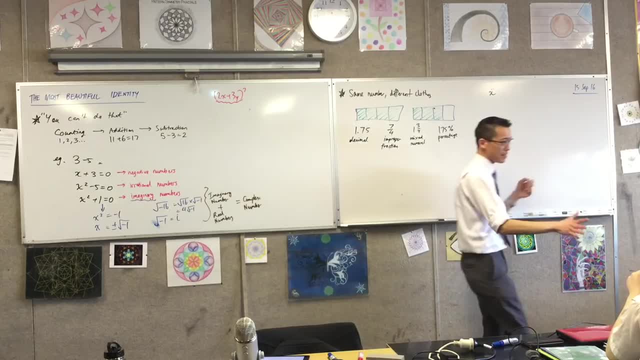 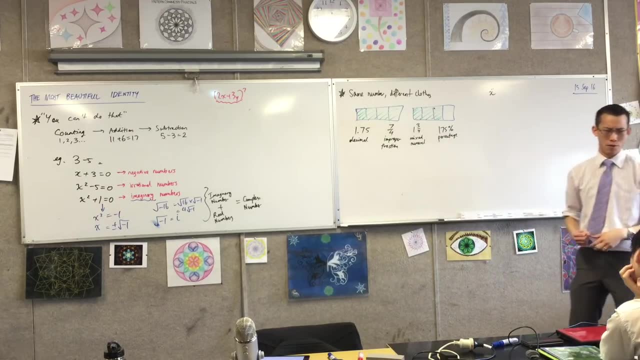 Example percentages. This would by far be the easiest if you wanted to describe like relative growth. I used to be this and now I'm this: Like 135% increase in profits over the last calendar year. something like that, right. 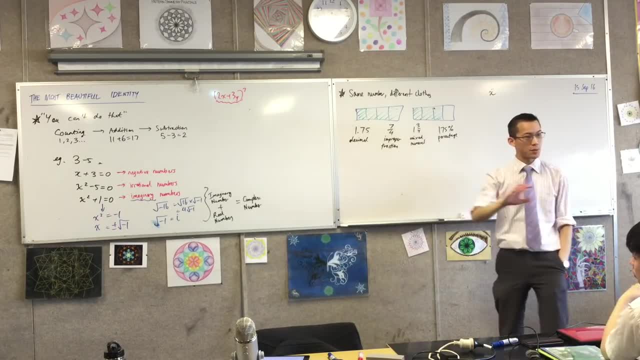 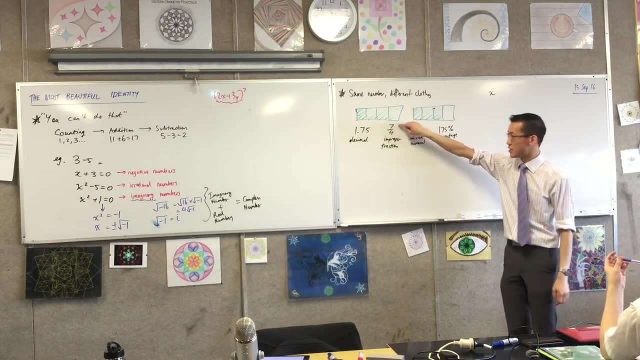 If, alternatively, maybe you wanted to describe a difference between a comparison of quantities, right Like ratios between two things, Well, clearly this is the best one, right? Seven? one of them's got seven and one of them's got four parts. okay. 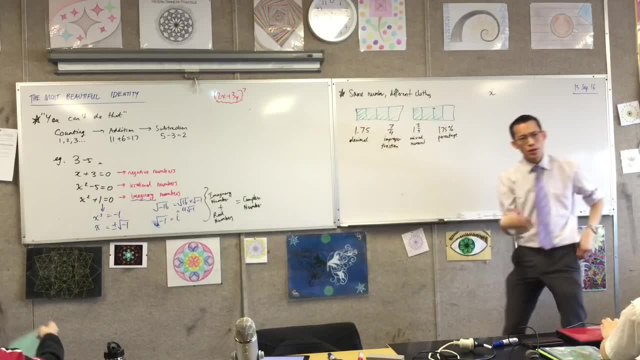 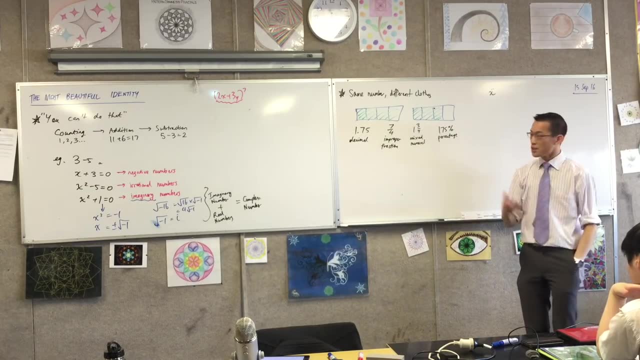 That's fine, right, If I was comparing this to this. So each one of these has a different kind of purpose that it leans toward, And complex numbers are the same. okay, So I'm going to show you- and this is where the extension- two people are going to end and we're all going to be in new ground. 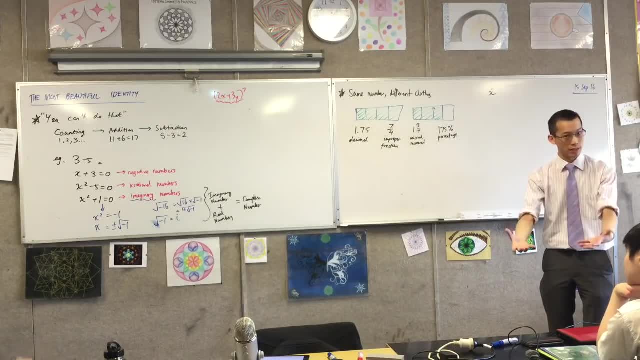 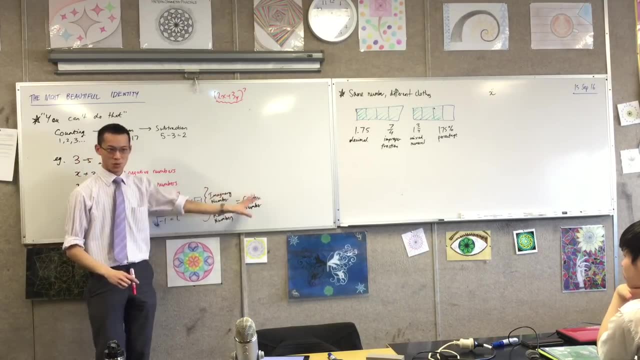 I'm going to show you the different ways we can write. visualize a complex number. okay. Now to help you with that, I want you to think back to these guys right Before we got to combining this with square root of negative one.